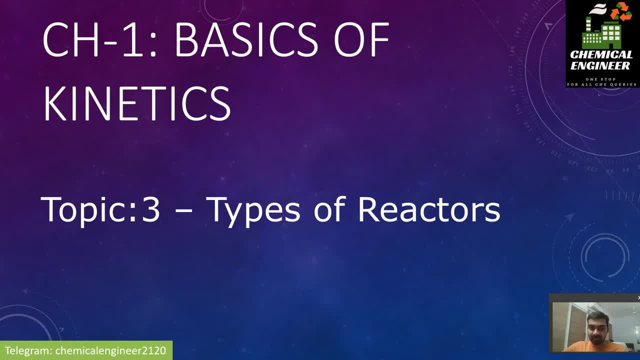 hello everyone. welcome to the channel. chemical engineer. I am Sahil Yadav and we are covering our course on chemical reaction engineering. so we are doing our first chapter, that is, basics of kinetics. so this is actually the base for chemical reaction engineering. we will be starting with our topic number three of 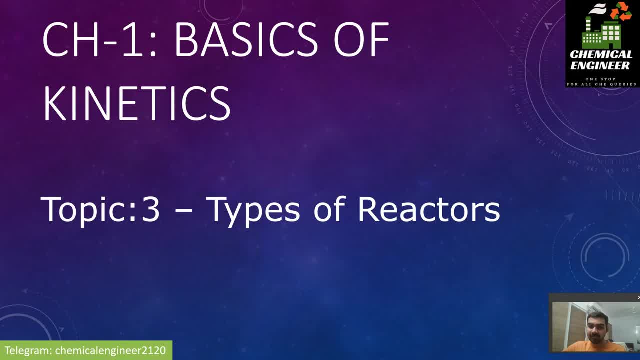 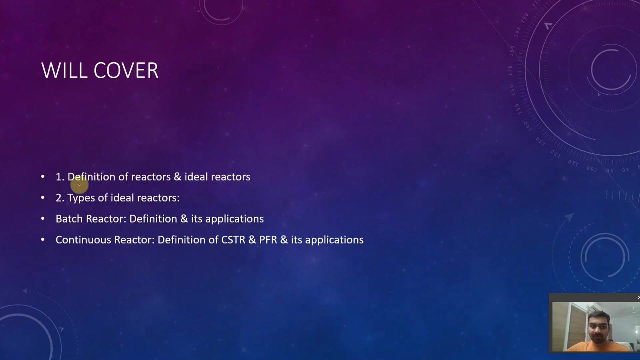 chapter number one, that is, types of reactors. so before starting the video, I would encourage you to subscribe to my youtube channel as well, as please do join our our telegram channel as well. okay, so let's start the video. so in this video, I will be covering four topics, that is, I will be covering about 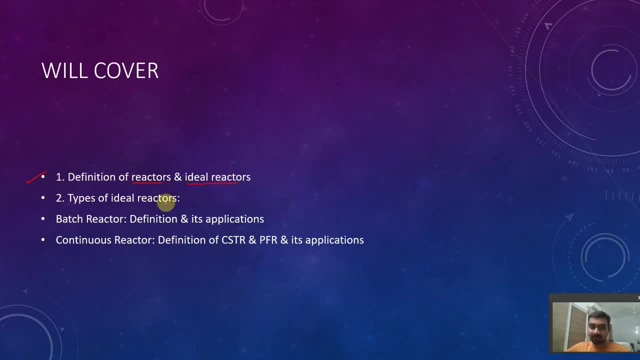 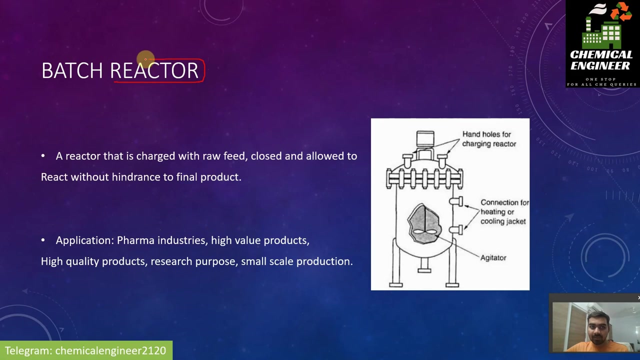 definition of reactors and what are ideal reactors. then we will see the types of ideal reactors. that is batch and continuous with its definition and its application. okay, so these all things we will cover in this 10 to 15 minute video. so reactor, okay, so what our aim is to design a reactor in CRE, chemical reaction. 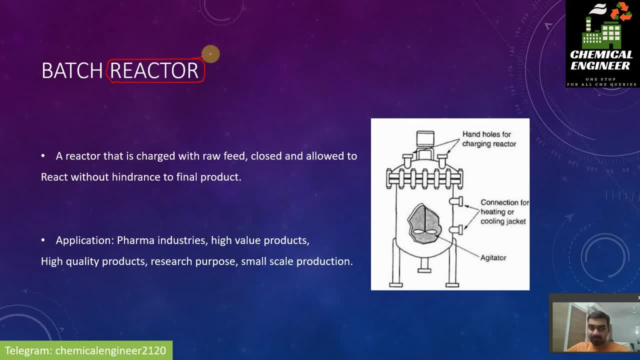 engineering, we aim to design a reactor. in CRE, chemical reaction engineering- we aim to design a reactor. so what is reactor? so reactor is nothing but a place or equipment where chemical reaction happens. chemical reaction occurs. so it is nothing but a place where chemical reaction occurs. okay, so that thing is. 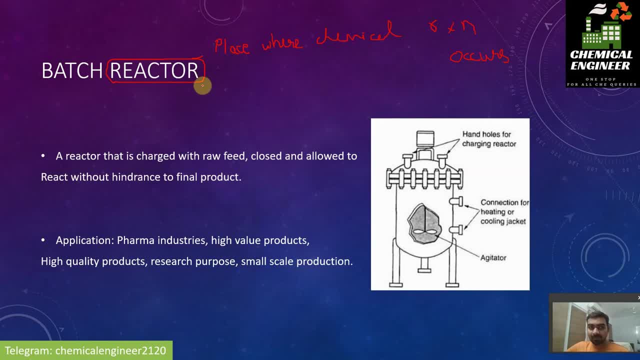 known as reactor. okay, and what are ideal reactors? so reactors which can be defined by using, or which can be designed by using, rate equation. okay, rate equation are known as ideal reactors. so those reactor which can be defined or which can be designed using rate equation, they are known as ideal. 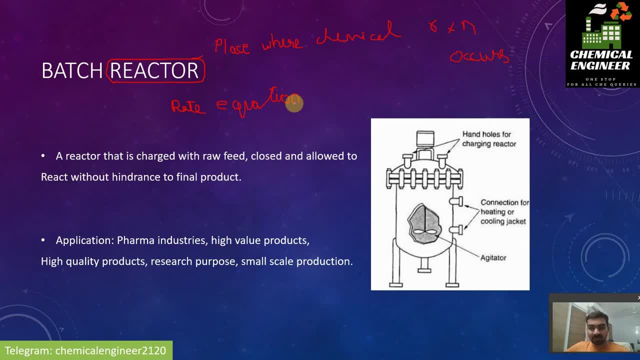 reactors in general. we have two types of ideal reactors. first is a bad reactor and second is a continuous reactor. so in this slide we will see about bad reactor. so, as the name suggests, batch, that means you have something confined in one space, what you do, that is called as a batch, like suppose i have a batch of chocolate. we can say so that. 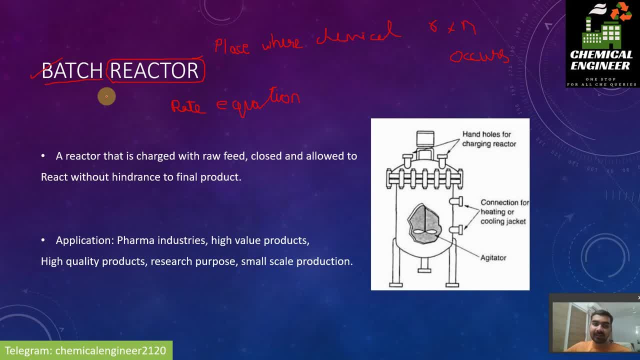 includes a box of a chocolate, is we can call it as a batch. okay, so those reactors which are having inlet from some point of a raw feed which is then closed, like once we feed the reactor we close the inlet. okay, so once we feed it using these two points, we will close these two points. 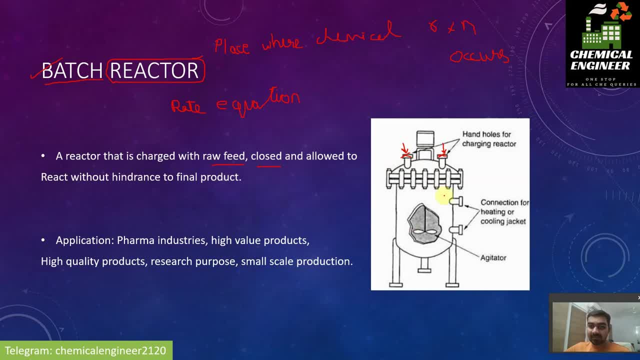 and then whatever thing is inside the reactor, we call it as a batch, we close it and we give it a time for reaction, okay, and then we have a place to take out the final product. these two are the places. so we open, these two places to take out the 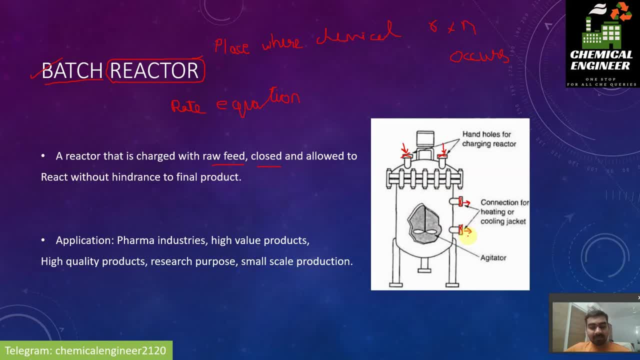 product. so what we can say? this is called batch reactor. we have one inlet, one outlet and a reaction in a reactor which is a batch reactor. batch reactor may have this agitator as well, as it may have a simple vessel. okay, so these two things may be there. so this type 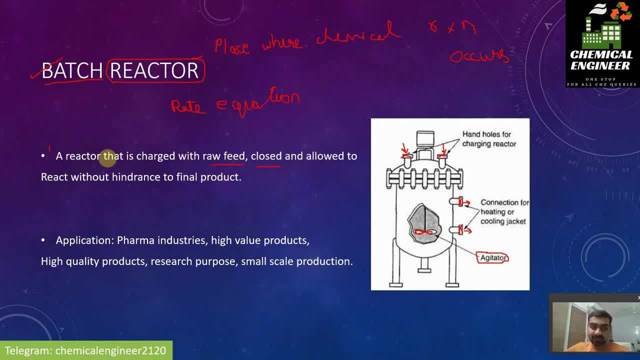 of reactor are batch reactor. so to define batch reactor: a reactor that is charged with raw feed, closed and allowed to react without any hindrance. two, a final product. this type of reactor are known as batch reactors. this is not for our case. okay. so the application of batch reactor is: they are used in pharma industries. they are. 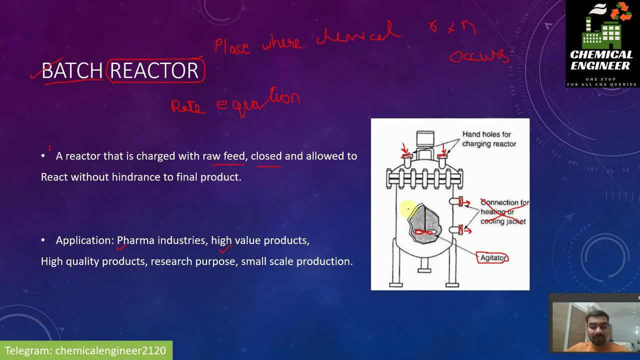 used in high value products, so in batch reactor. you should have clear idea that we will be using batch reactor only to the places where we need high quality products. okay, so high quality product, So for a high value product- means high costly products, then we can use this reactor for. 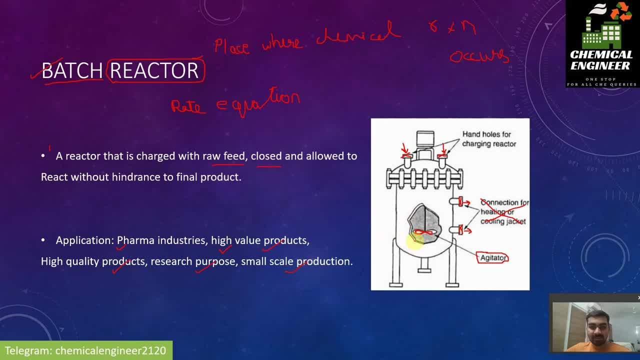 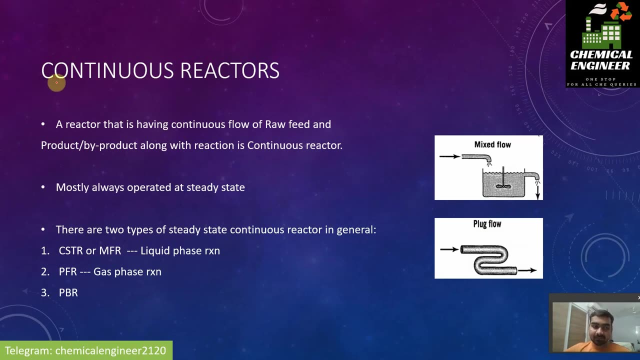 research purpose or for small scale production, because material takes much time for reaction. okay, so this is all about batch reactor. second type of reactor that we have is continuous reactor. so, as the name suggests, continuous means there is no holdup like in basilikat. this means that the previous method to burning of linear Baak- since this is内 lopед- 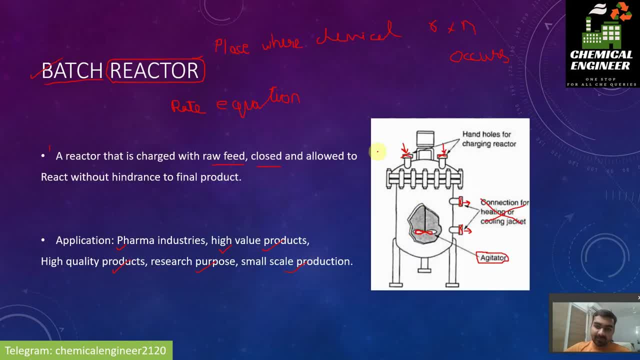 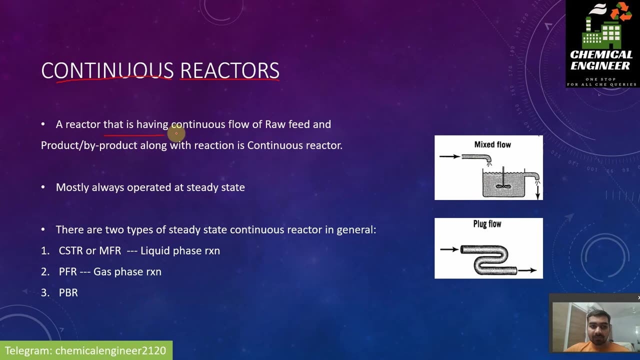 the Como example We can use Class dedication R also means seal. that to forget about filling up tough pressure boys reactor. we have to fill the tank, then hold it for reaction and then we take it out. but in this continuous type of reactors we don't hold the product. what we do, we have a continuous flow of 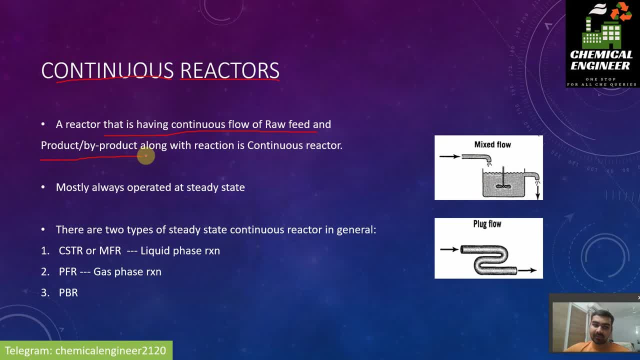 a raw feed and by product or product. so there are two type of batch reactor- continuous reactors. and for our study in chemical reaction engineering we will be assuming that this continuous reactor is operating at steady state. steady state means parameters does not change with time, so parameters does not change with time. so those type of reactors are steady state reactors. 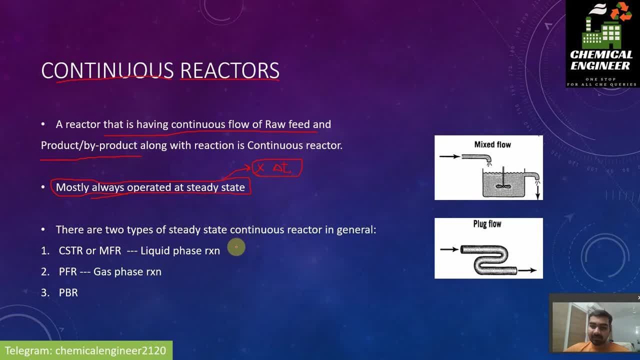 there are two types of, or we can say three types of reactors. so first is chdr or we can say it as mfr, second is pfr and third is pbr. so you may be asking: what is the full form of chdr? what is the full form of mfr? 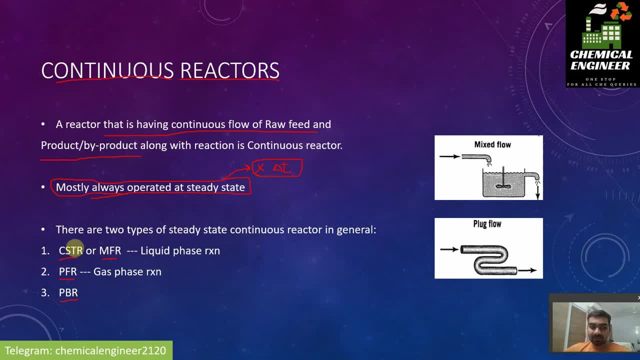 so i would recommend you to please write it down: chdr is having a full form of continuous, continuous stirred, continuous stirred tank reactor. okay, so full form of this chdr is continuous stirred tank reactor, which is also known as mixed flow reactor. okay, so there are two names for chdr. it is also known as mixed flow. 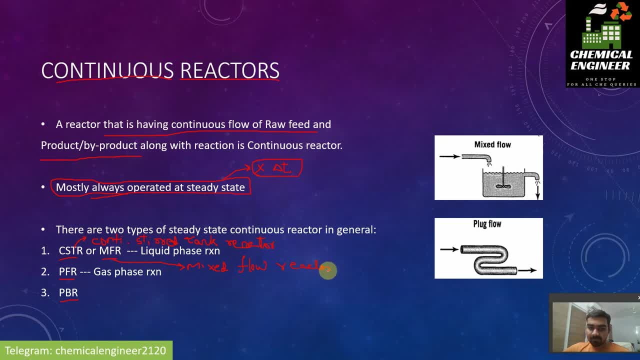 reactor. so what happens in this type of reactor? this is a schematic. we have one inlet going to the reactor. this is a reactor and it is having a continuous outlet. so here what will happen? the product will go to the bottom, it will react in this meantime and then. 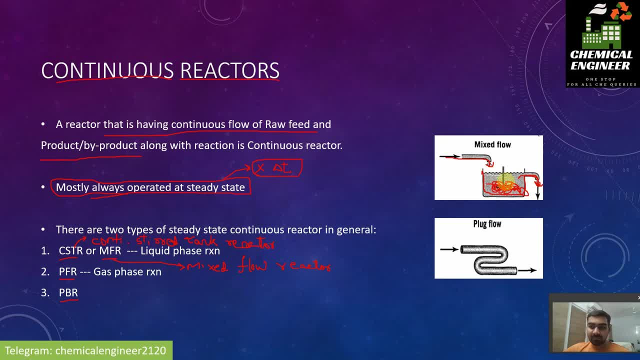 comes out, so this is a continuous operation. there is no valve or something like that, so this is continuous operation and in chdr we generally have agitator. okay, so this agitator is generally a representation of chdr and this is how we represent chdr, that is, having a vessel with 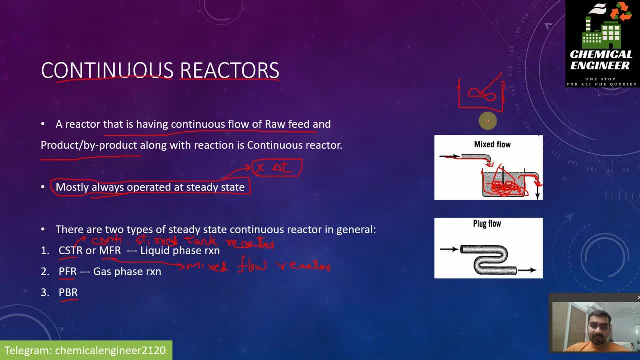 agitator. okay, so this is all about mfr. second, we have pfr, which is known as plug flow reactor. these are the pipe type reactors. okay, so tubular reactors, or pfr, that is, plug flow reactor, those are the reactors which are generally used for gas phase. 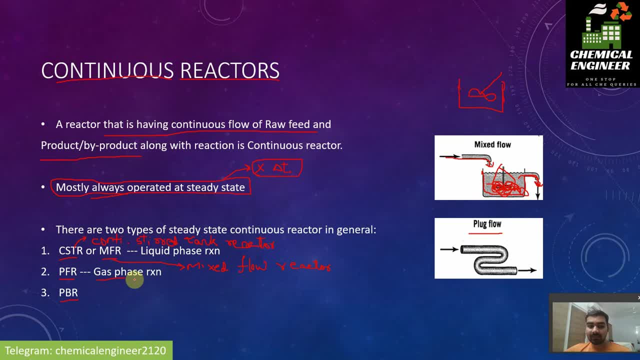 reaction and they do generally have axial mixing. axial mixing will be there in tubular type of reactor. and then, third, we have a packed bed reactor. so packed bed reactor is nothing but a reactor which is having a packing of something. so this is how we define it: packed bed reactor. they are generally used for liquid.